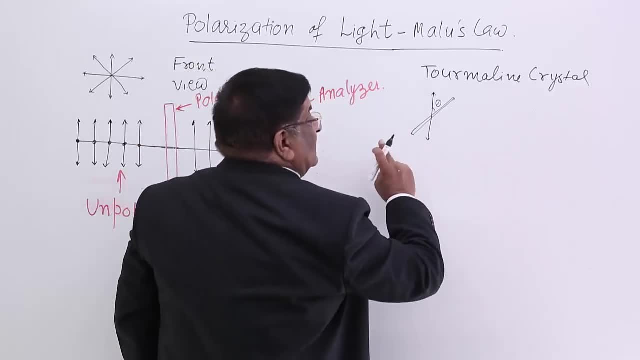 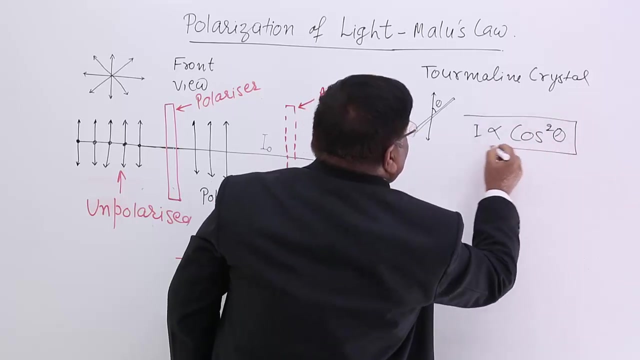 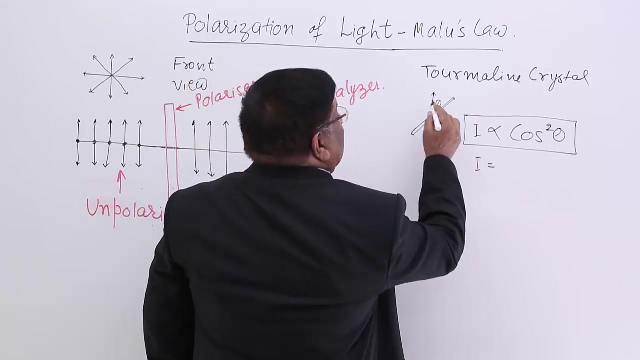 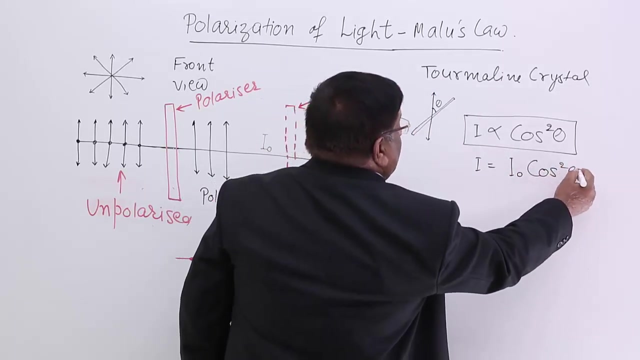 its intensity of light and that intensity, what is reaching me, that intensity is proportionate to it, is related to theta and that intensity is proportionate to cos square theta. If a constant is to be put here, that constant is The maximum intensity this polarized light was having: I0 cos square theta. This relation. 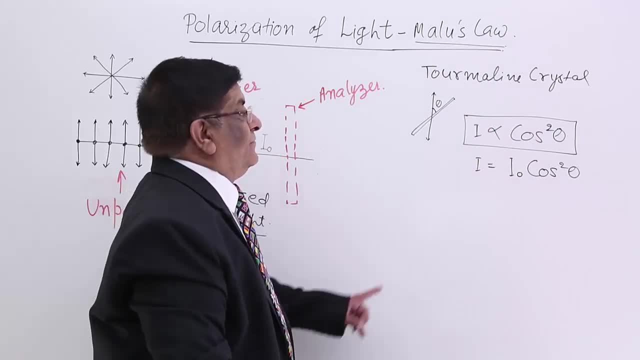 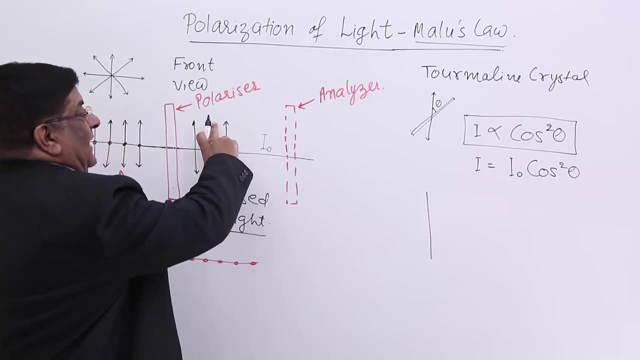 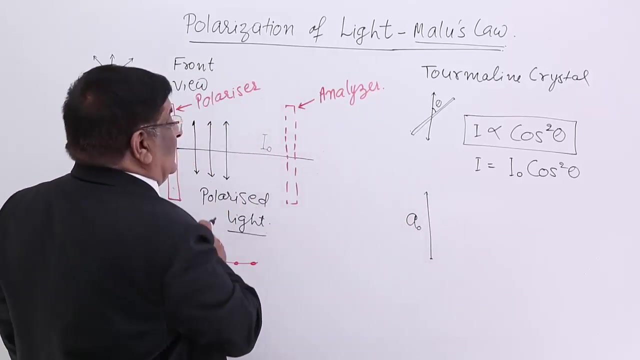 is known as Marlowe's law. See, here is amplitude of this light. This amplitude is A0, which gives us the intensity. So this is the intensity of the light, This is the amplitude of the light, This is the expression of the hö descrição of theibel light, the intensity of this light. This образом, 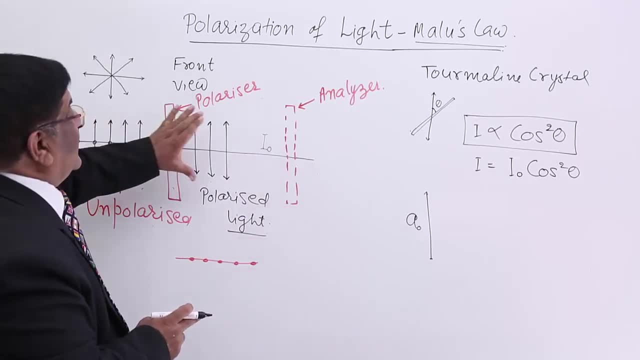 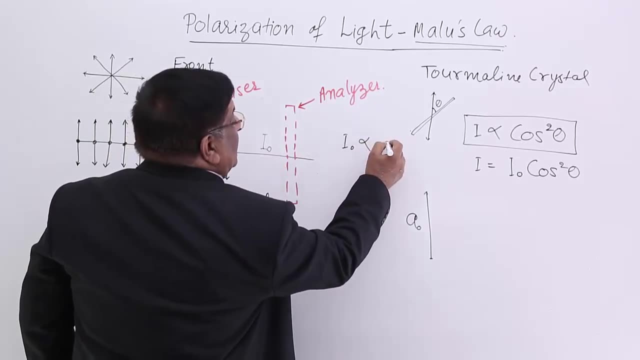 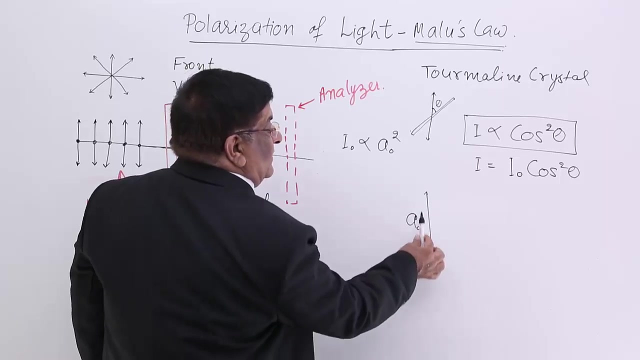 is required. So we have this. We have thisиком формatreadn New Marlowe's law. We are discussing the intensity of the照 of the nutrient. So we have a new, rather verbatim function which is going to represent the intensity. 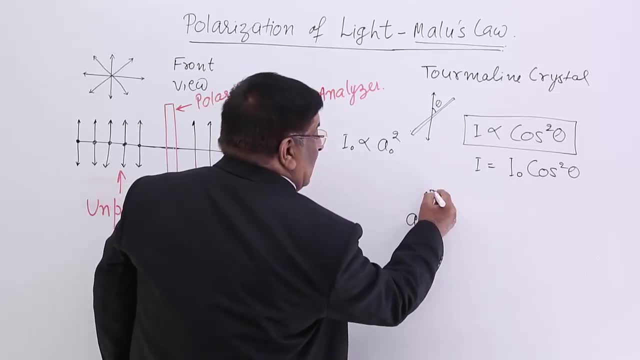 the intensity of this light, The full intensity of the polarized light. We are not discussing unpolarised, We are discussing only polarized. So it has got intensity I0 and we know I0 is this. then it will pass through this A0 will pass through this. Now, if I turn this window, 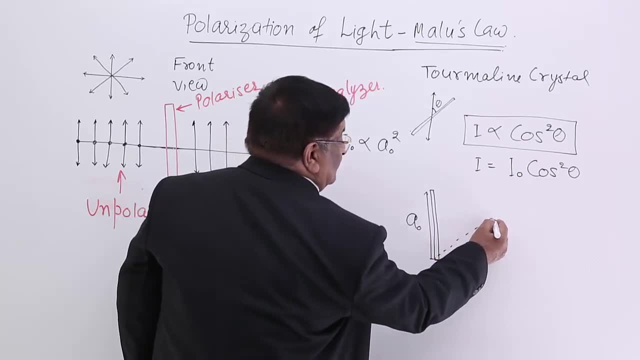 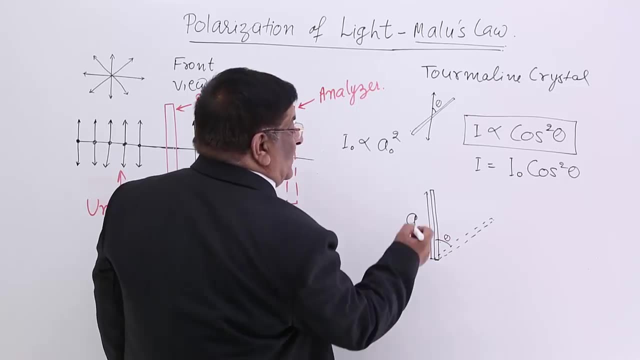 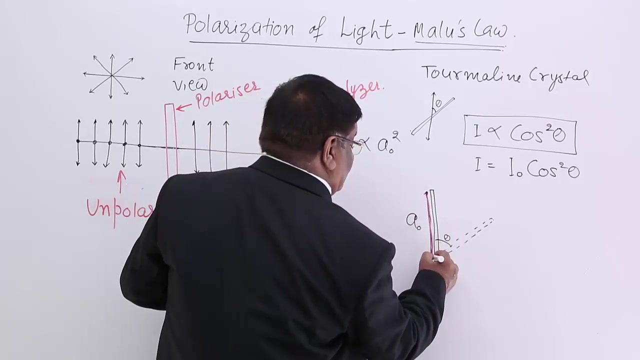 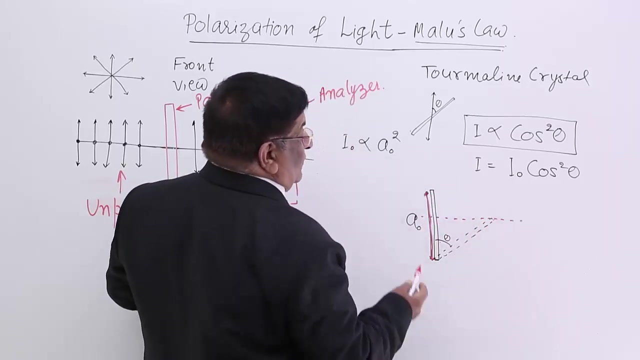 by theta degree, then this window will be here, this direction turn by theta degree. Now what happens? that this amplitude, that is this vibration which is moving in this direction, it keeps on moving. You will see this much portion here to here this much. 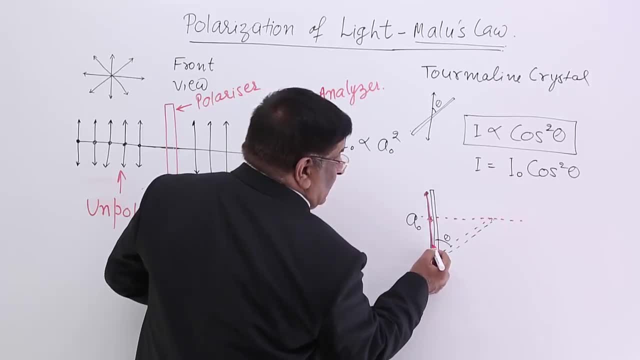 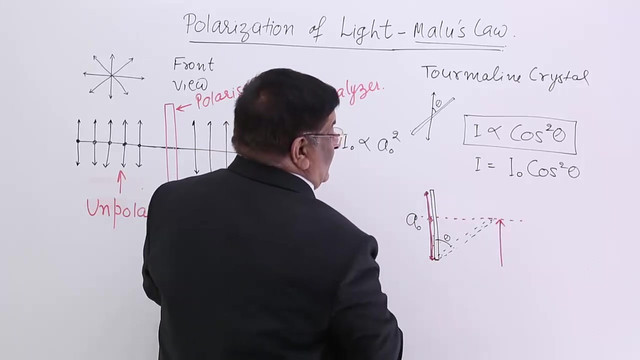 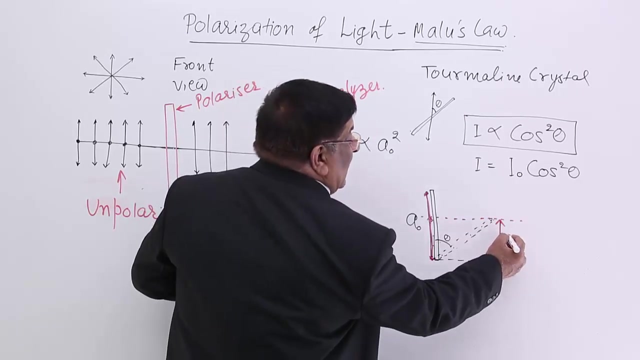 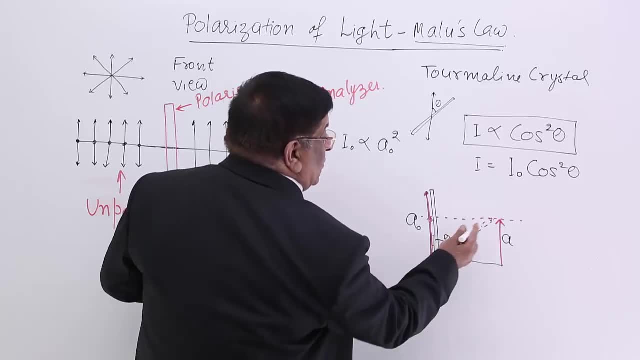 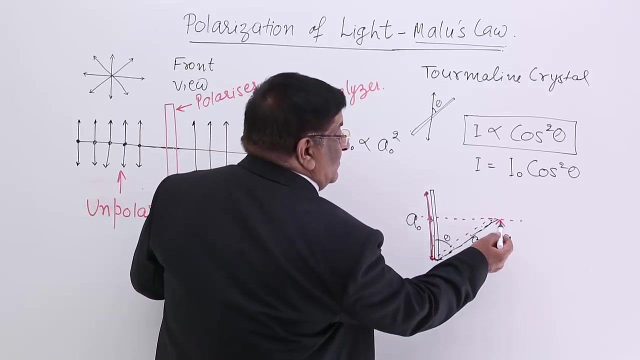 size A0 has been turned like this. so how much is this length? So this length is the center of a bar. So this length is the center of a bar. So this length is the center of a bar, same length which is turned. this is A0, okay, Now this is amplitude of the light, which. 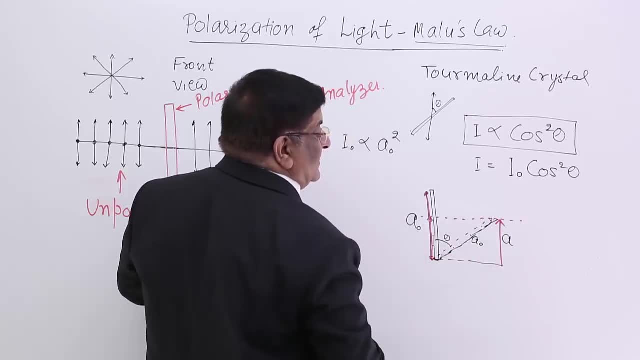 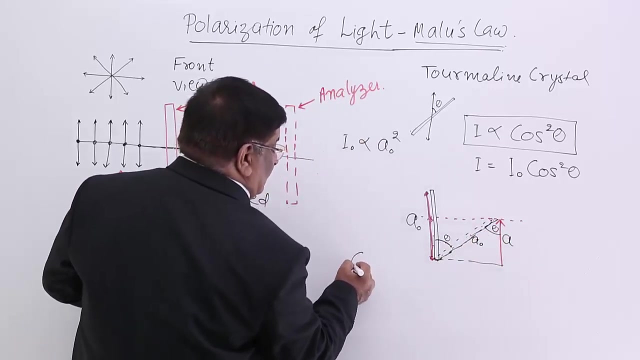 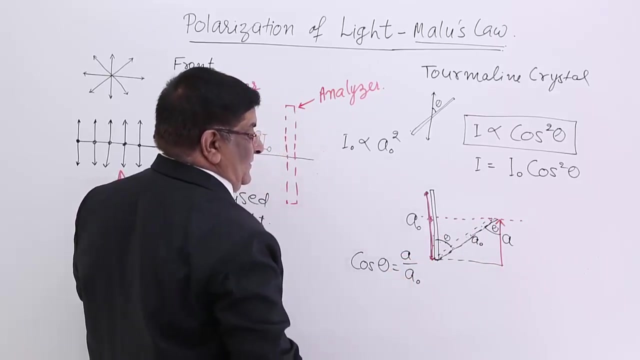 has passed through the crystal slit and this size is A0, this angle is theta- turning angle- and by geometry, these are two parallel lines. if this is theta, this is also theta. Now, what is cos theta here? Cos theta is equal to base upon hypotenuse A, upon A0, okay, Make. 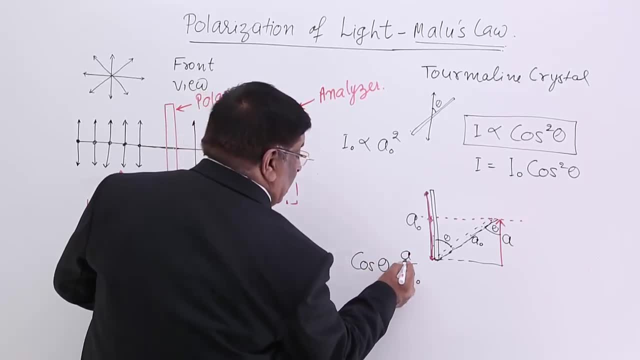 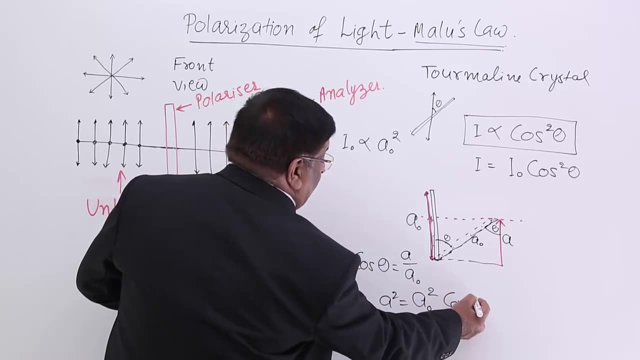 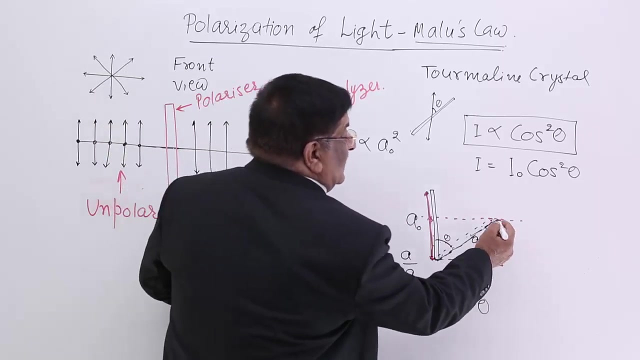 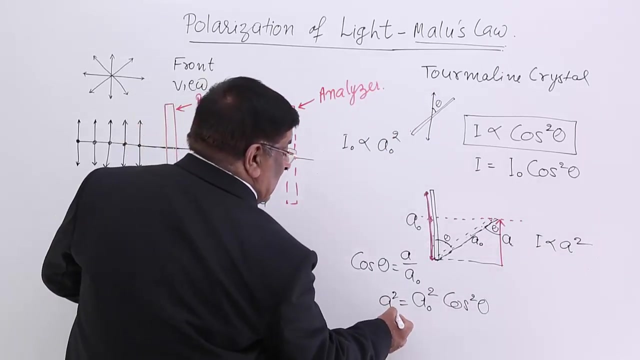 the square of the two sides. so this will be A square is equal to A0 square cos square, theta. Now you know, I0 is proportionate to A0 square and what I see here, intensity of light, I, That is proportionate to A square. so here I can write it: I is equal to A0 square I0. 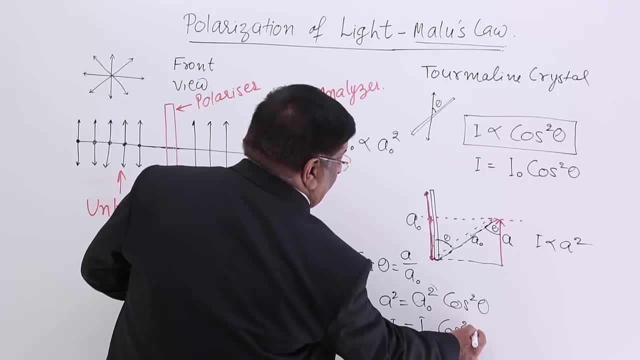 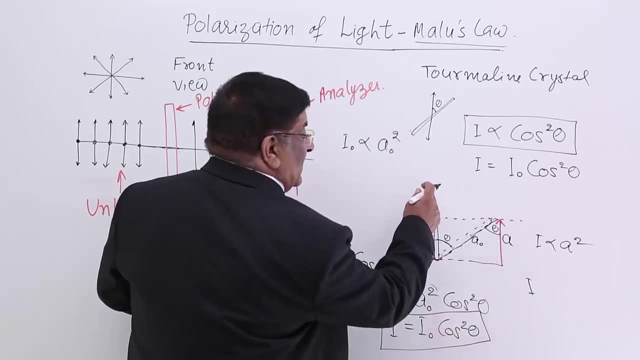 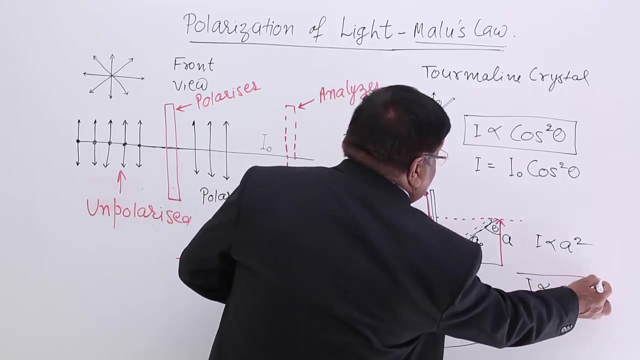 I0 and this is cos square theta. So I is equal to I0 cos square theta, and simply I0 is a constant, the full value. Therefore I can write it: I is proportionate to cos square theta. what is theta? Theta is the angle by which we are turning the analog. 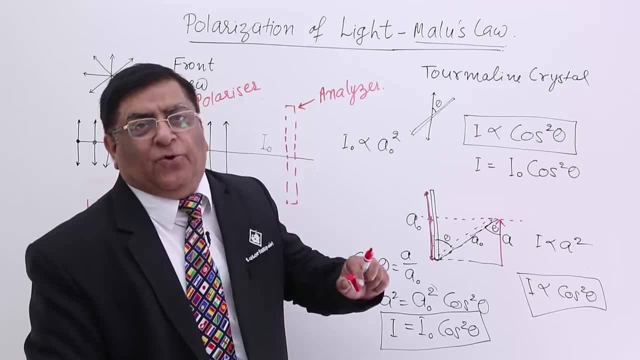 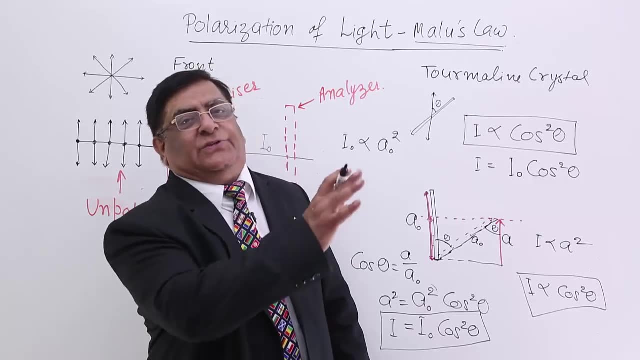 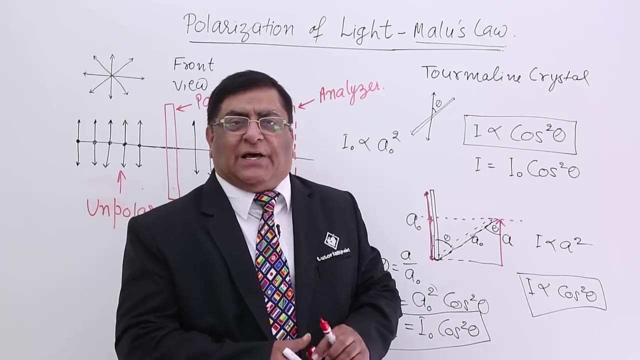 So if we turn it by full 90 degree, then cos 90 is equal to 0 and we will not be able to see the light. This is Marlowe's law. Now, with Marlowe's law, sometimes it is asked what should be the angle which make the intensity. 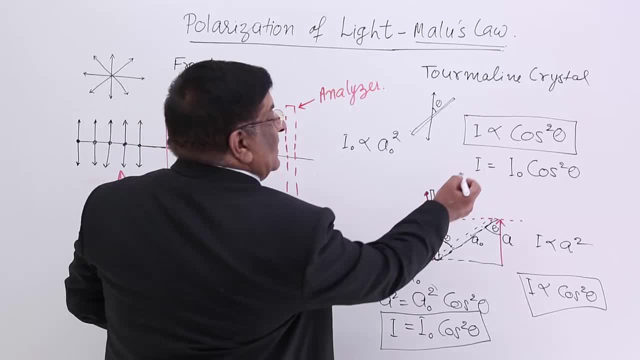 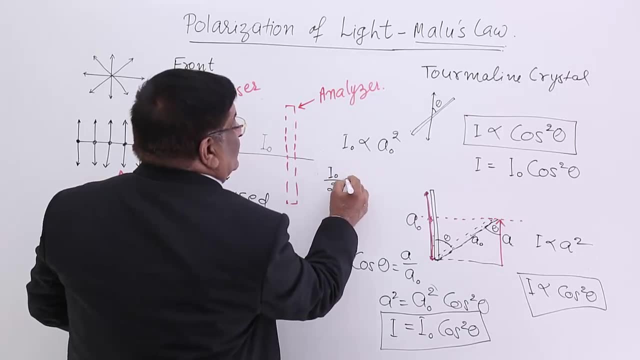 half. So we will write: I is equal to I0 cos square theta. the intensity has to become half, that is, I0 upon 2.. This is equal to I0 cos square theta and this gives us cos theta is equal to 1 upon root.